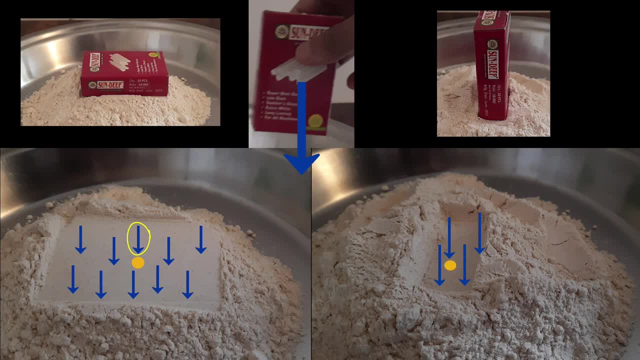 on the right, the amount of force that appears or acts on any one point of the flour is larger. So if have the same force, then the depth of the mark is less when the box was kept horizontal and the depth of the mark is more when the box was kept vertical. It matters how concentrated the force. 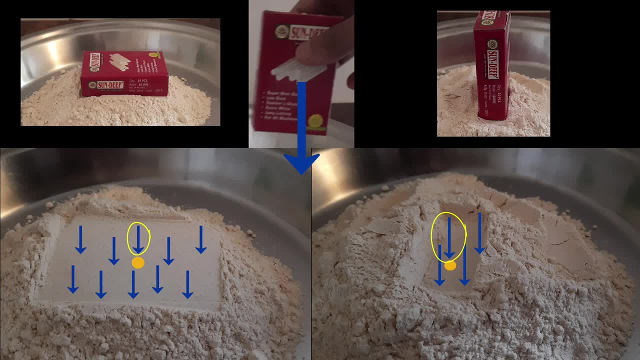 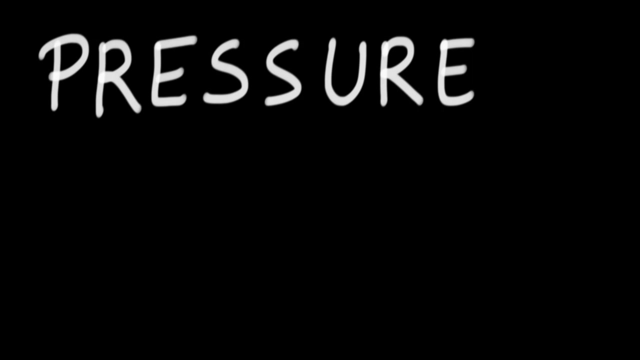 is Same force is divided over a larger area in the first case, so it is not that concentrated. but when the same force is divided over a smaller area, then it is more concentrated, and this is what we call pressure. Pressure can be thought of as how concentrated your force is. We can even 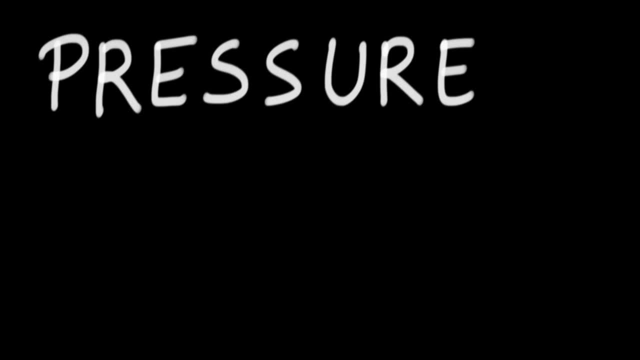 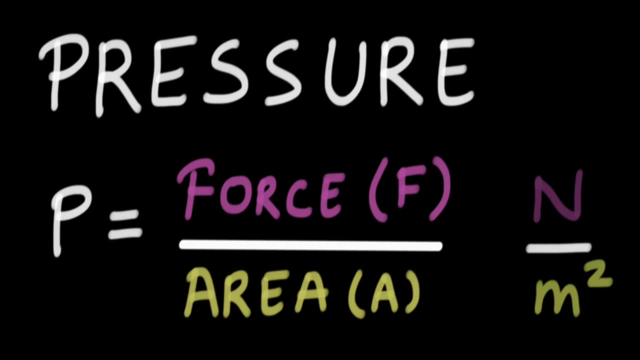 calculate pressure. Well, just like we saw that, we are basically calculating how much force gets divided over the area. mathematically also, pressure, that is, p, is calculated as the force divided by the area and its units will be newton per meter square. So in the first case, when the area was 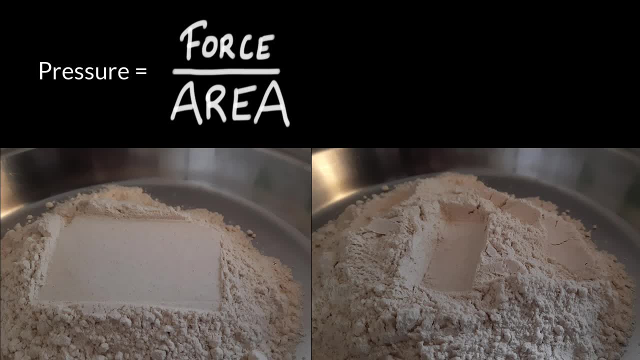 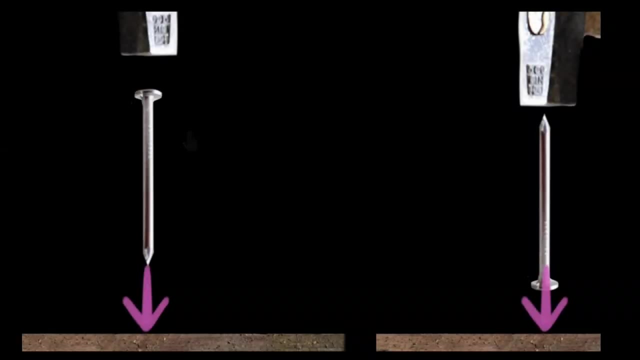 very large, The pressure was small. but in the second case, when the area was small, the pressure became large. Now let's come back to our original question. Why do we hammer a nail with a pointy end at the bottom? Well then, force is concentrated over a very tiny area, but in the case on the right, the same force. 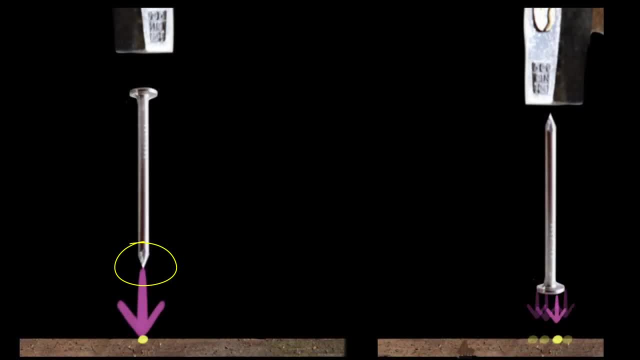 is concentrated over a larger area and, as a result, if you now compare the amount of force that appears on the same space, So the force that appears on the same spot as before, the force has reduced a lot. right, Because it got divided. The contact area was very small in the first case, so the pressure was very 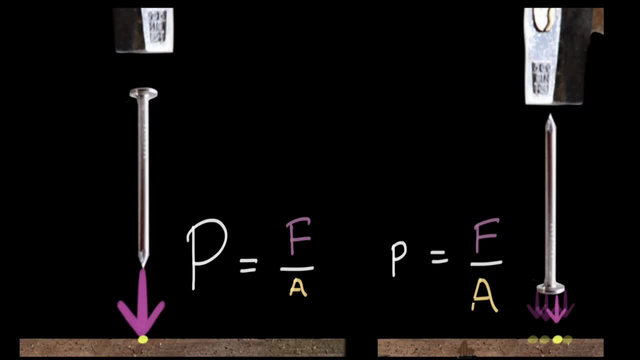 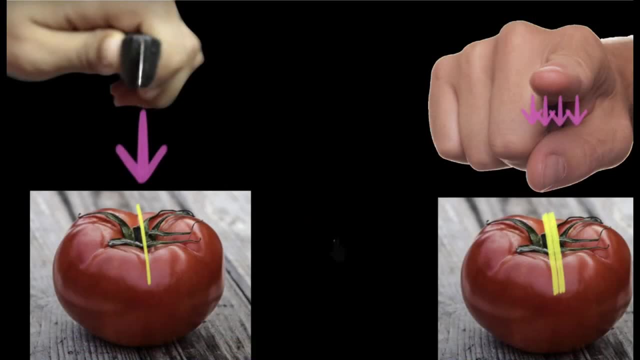 high and the contact area was large in the second case, so the pressure is very low. Similarly, when you use a knife and put a force, then all the force gets concentrated into a very tiny area. The tip of the knife is very sharp, So that means the tomato experiences a large pressure. but